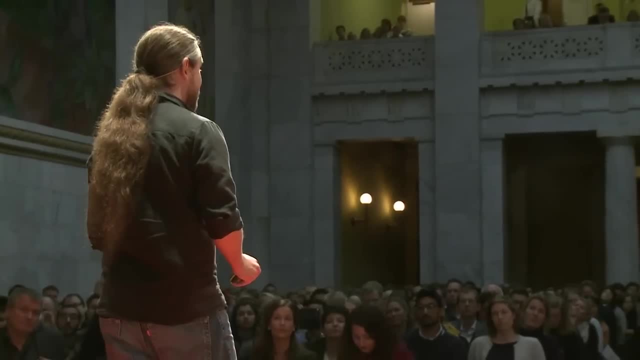 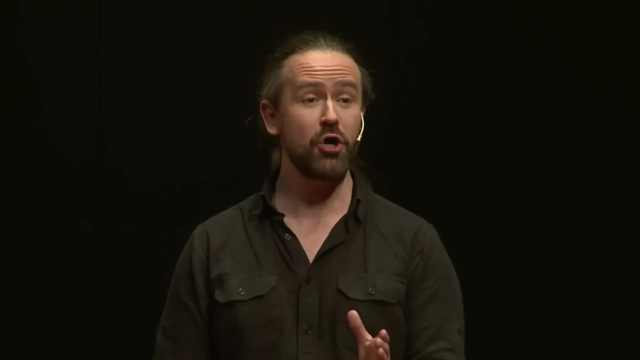 I want to talk about the essence of mathematics as well, And my claim is that mathematics has to do with patterns. Behind me you see a beautiful pattern, And this pattern actually emerges just from drawing circles in a very particular way. So my day-to-day definition. 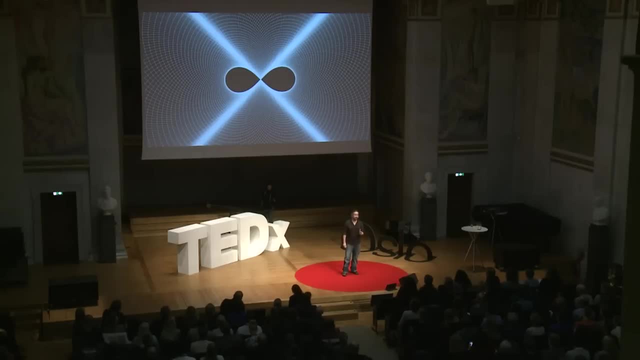 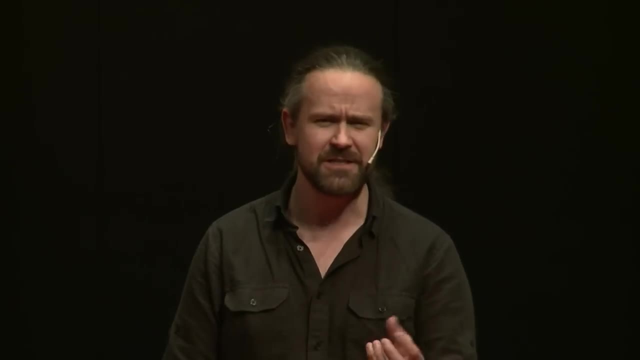 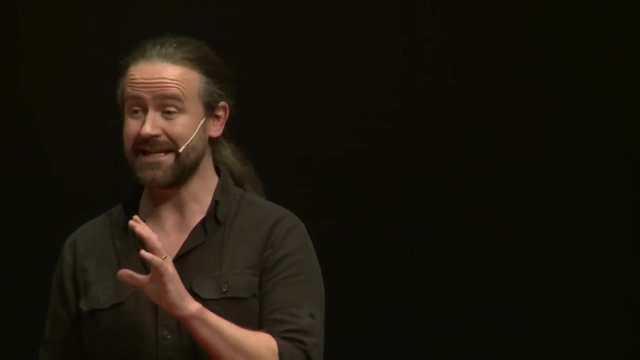 of mathematics that I use every day is the following: First of all, it is about finding patterns, And with a pattern I mean a connection, a structure, some regularity, some rules that govern what we see. Second of all, I think it is about representing these patterns with 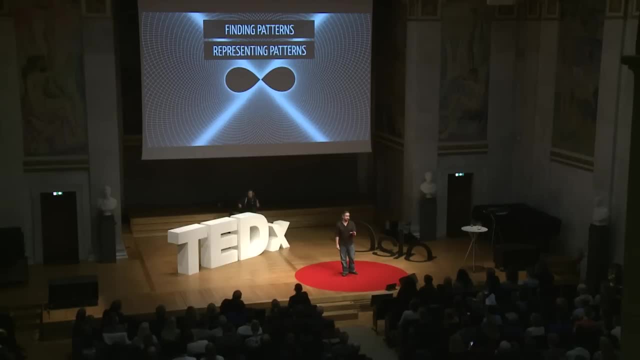 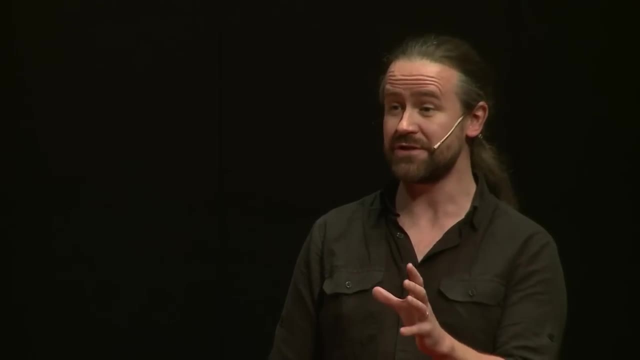 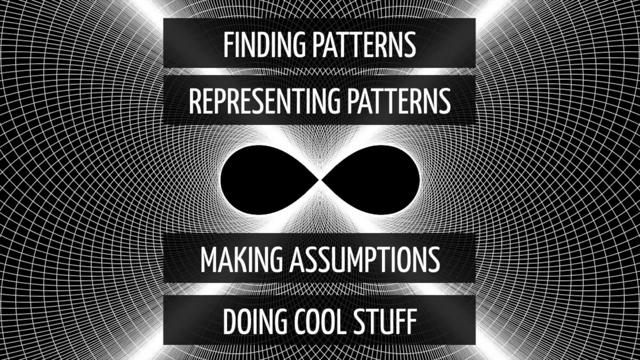 a language. We make up language if we don't have it, And in mathematics, this is essential. It's also about making assumptions and playing around with these assumptions and just seeing what happens, And we're going to do that very soon. And finally, it's about doing cool stuff. 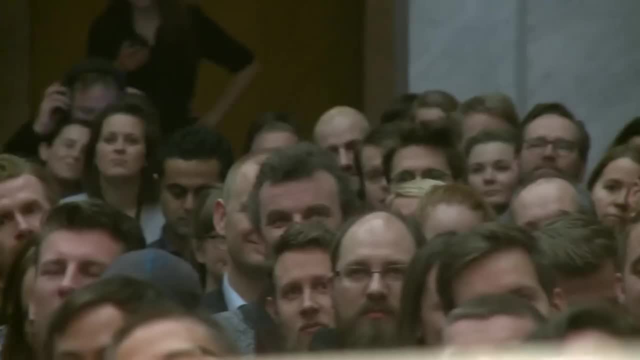 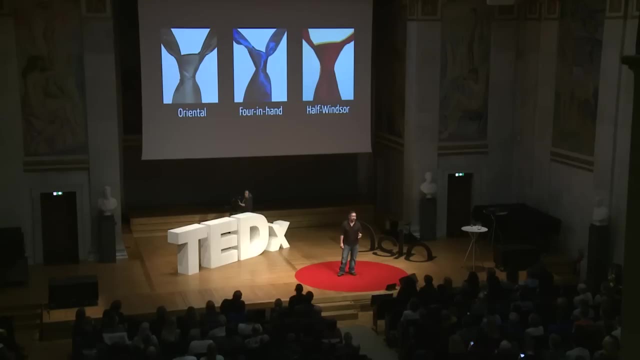 Mathematics enables us to do so many things, So let's have a look at these patterns. If you want to tie a tie knot, there are patterns, Tie knots have names And you can also do the mathematics of tie knots. This is a left-out, right-in, center-out and tie. 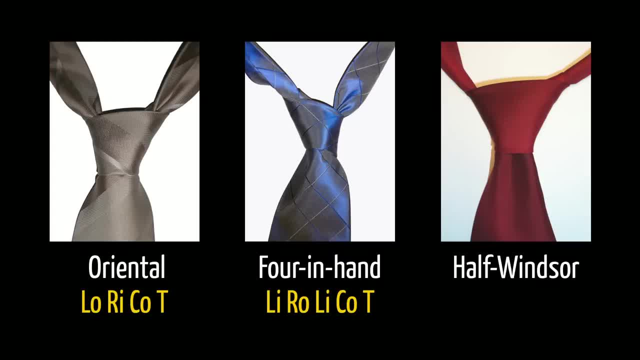 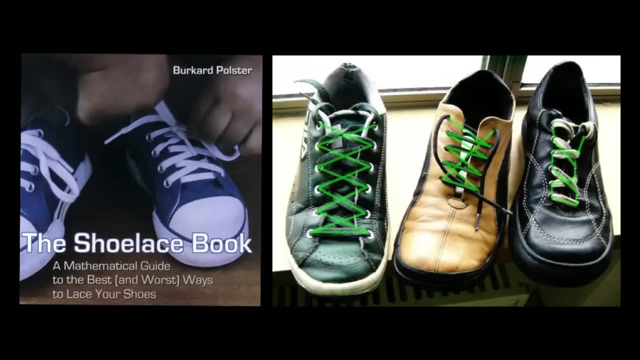 This is a left-in, right-out, left-in, center-out and tie. This is a language we made up for the patterns of tie, knots And a half-windthrow is all that. This is a mathematics book about tying shoelaces at university level, because there are patterns in shoelaces You can do. 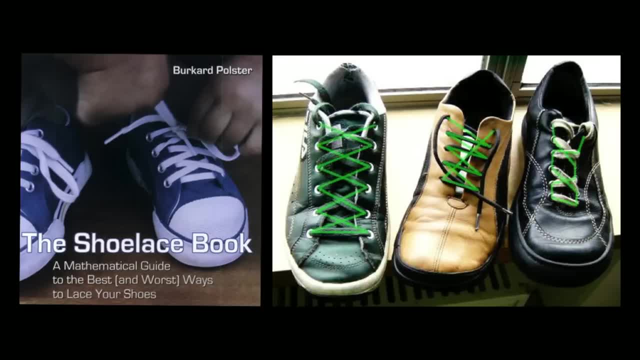 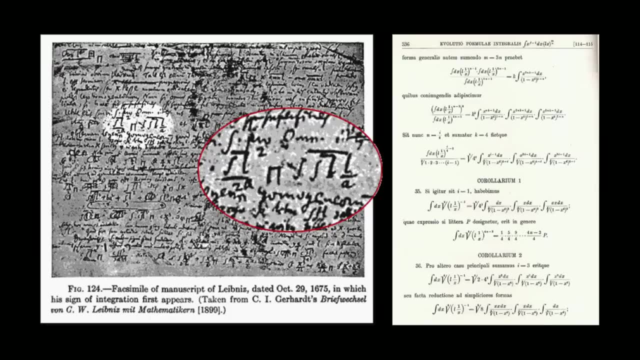 it in so many ways. You can do it in so many ways. You can do it in so many ways. You can do it in so many different ways. We can analyze it, We can make up languages for it, And representations is all over mathematics. This is Leibniz's notation from 1675.. He invented a. 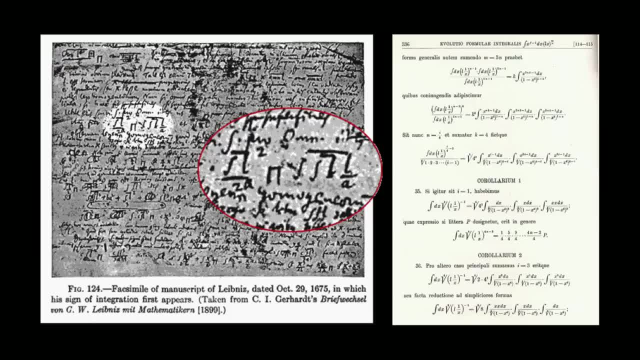 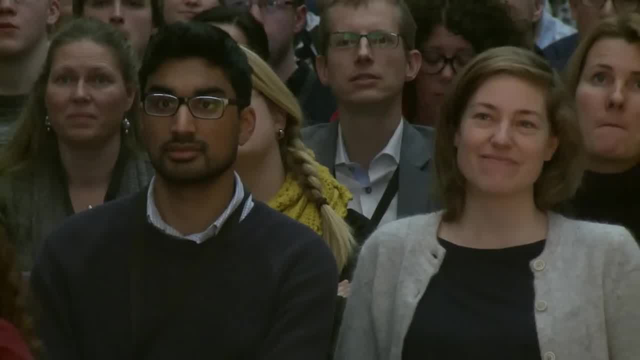 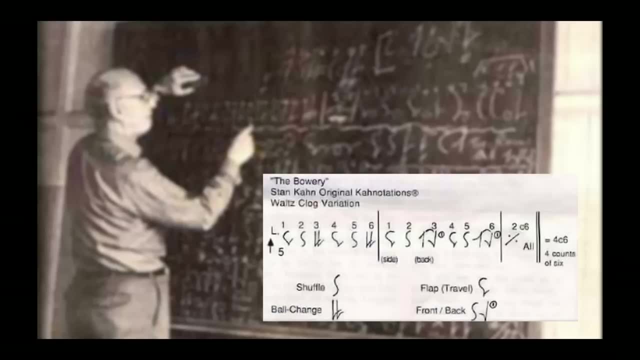 language for patterns in nature. When we throw something up in the air, it falls down. Why, We're not sure, but we can represent this with mathematics in a pattern. This is also a pattern. This is also an invented language. And can you guess for what? It is actually a notation system for dancing, for tap dancing. 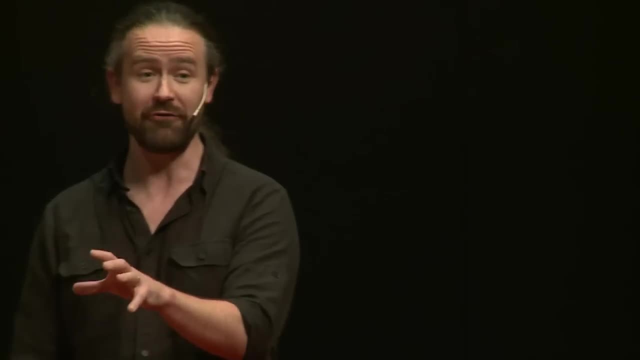 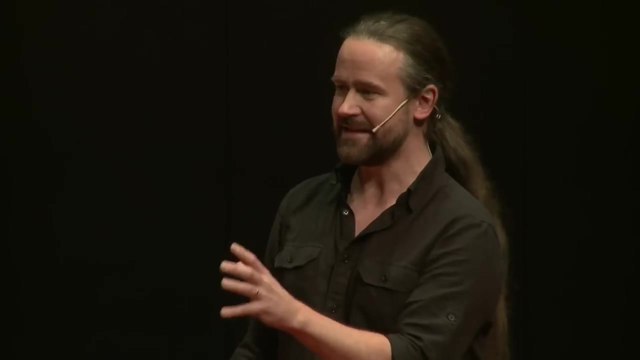 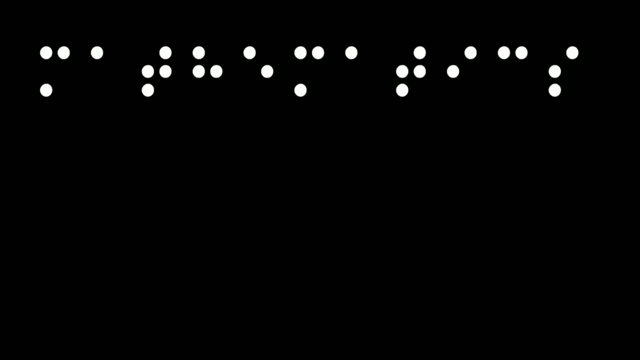 And that enables him, as a choreographer, to do cool stuff, to do new things, because he has represented it, And I want you to think about how amazing representing something actually is. Here it says the word mathematics, But actually they're just dots, right? So how in the world can 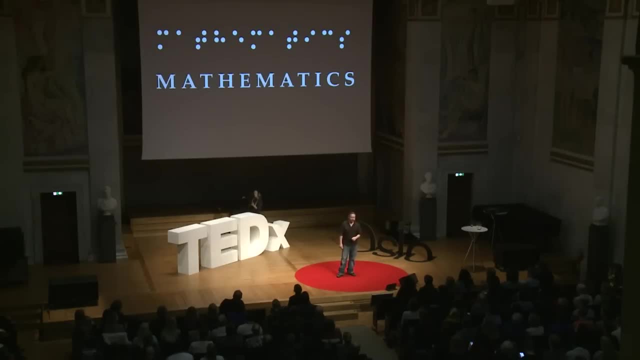 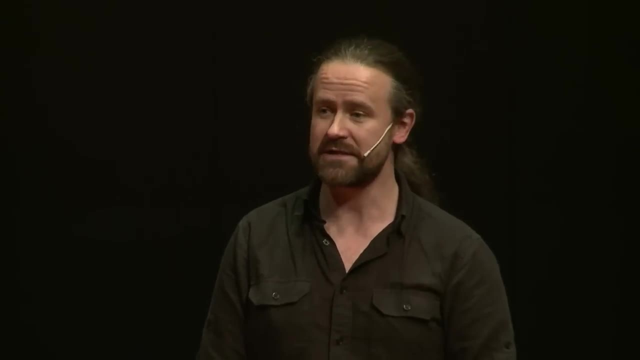 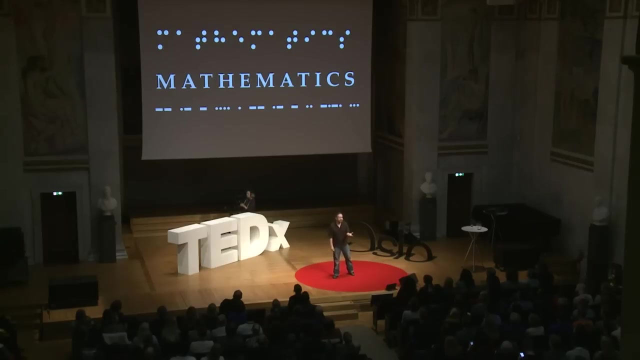 these dots represent the word? Well, they do. They represent the word mathematics, And these symbols also represent that word. And this we can listen to. It sounds like this: Somehow these sounds represent a word and a concept. How does this happen? And there's something amazing going on about representing stuff, So I want to talk. 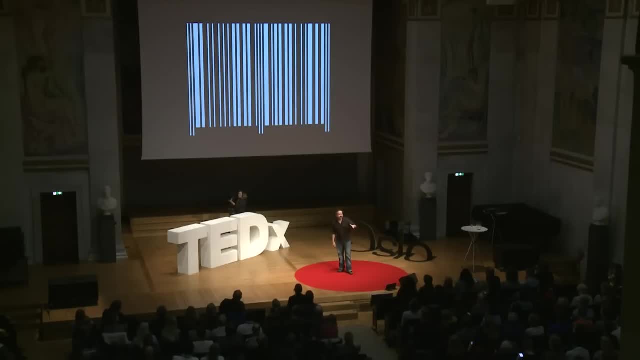 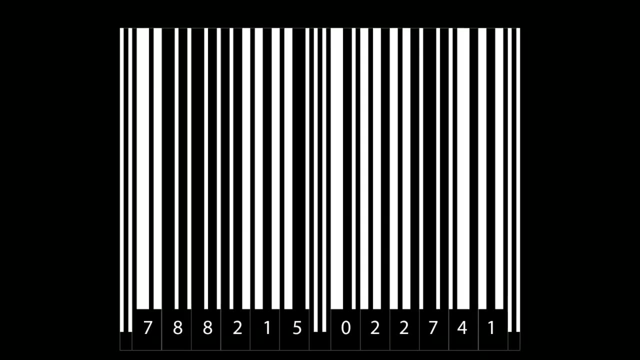 about that magic that happens when we actually represent something. Here you see just lines right And the numbers that we draw with. they stand for numbers for a particular book And I can actually recommend this book. It's a very nice book, Just trust me. 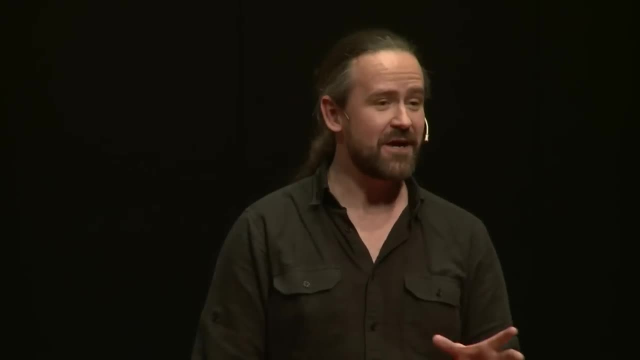 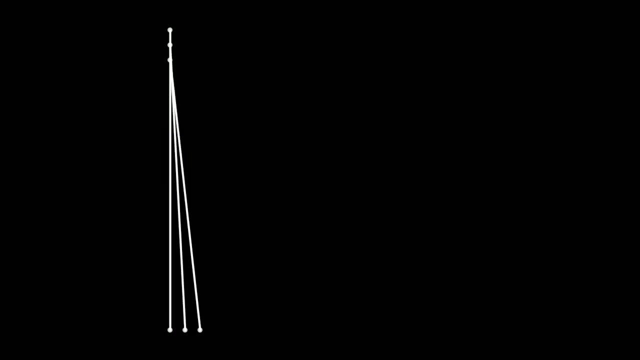 Okay, so let's just do an experiment, Just play around with some straight lines. This is a straight line, Let's make another one. So every time we move, we move one down and one across and we draw a new straight line, right. So we do this over and over and over And we look for patterns. So this: 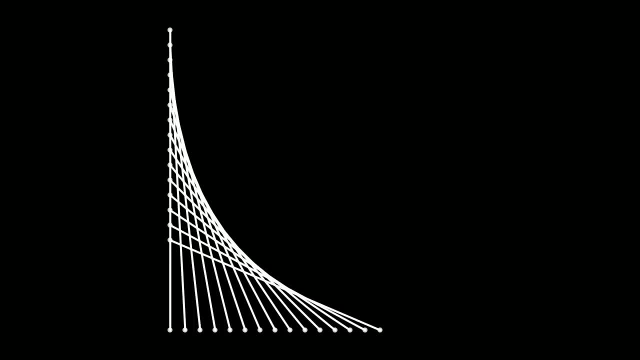 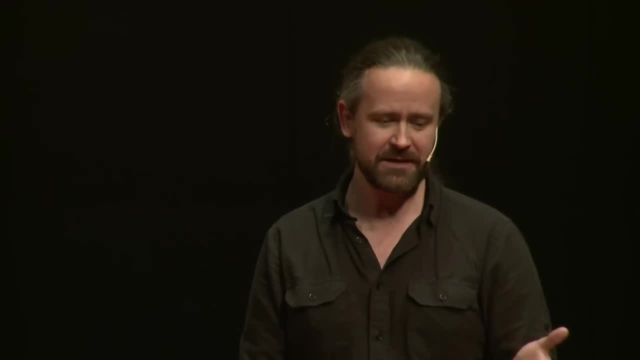 pattern emerges And it's rather a nice pattern. It looks like a curve right Just from drawing simple straight lines. Now I can change my perspective a little bit. I can rotate it And then have a look at the curve. You know what does. 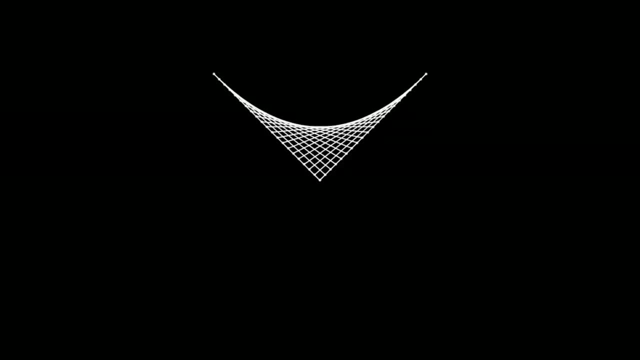 it look like, Is it a part of a circle? It's actually not a part of a circle. So I have to continue my investigation and look for- you know, the true pattern. Or perhaps if I copy it and make some art, well, no, Perhaps I should extend the lines like this and look for the pattern there. 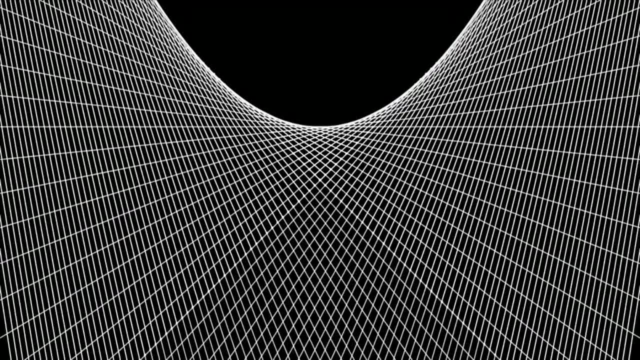 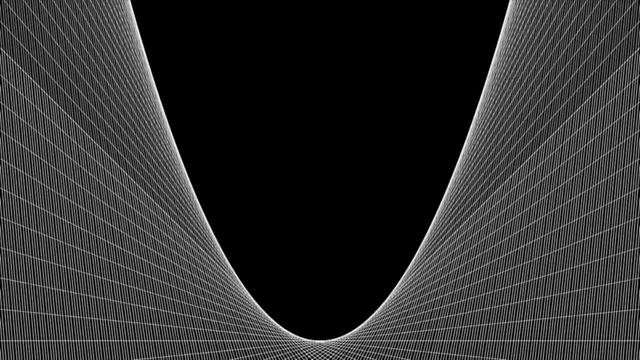 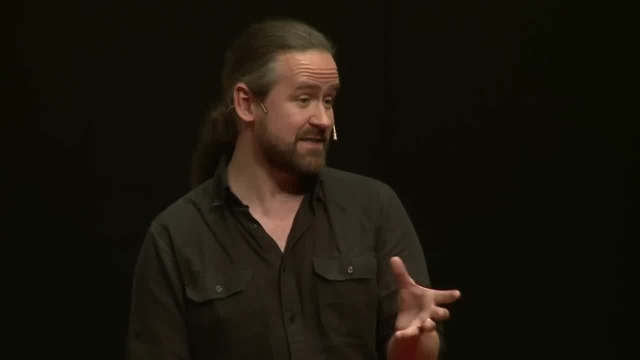 And let's make more lines. So we do this, And then let's just zoom out and change our perspective again, And then we can actually see that what started out as just straight lines is actually a curve called the parabola. This is represented by a simple equation and it's a beautiful pattern. So this is the stuff. 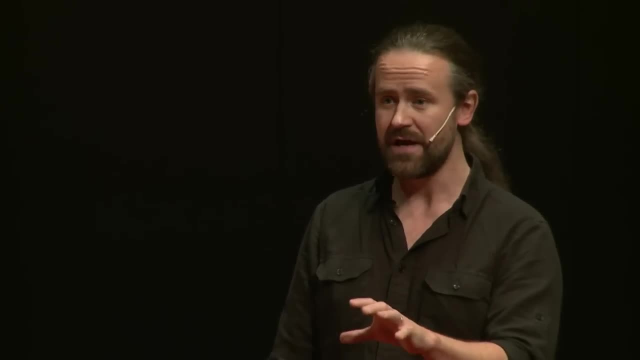 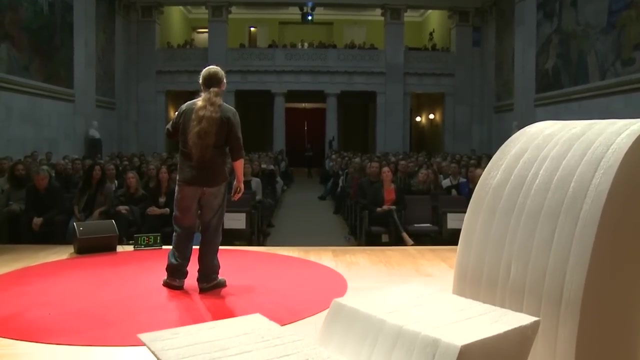 that we do. We find patterns and we represent them, And I think this is a nice day-to-day definition. But today I want to go a little bit deeper and think about what is the nature of this, What makes it possible? And there's one thing that's a little bit deeper and that has to do. 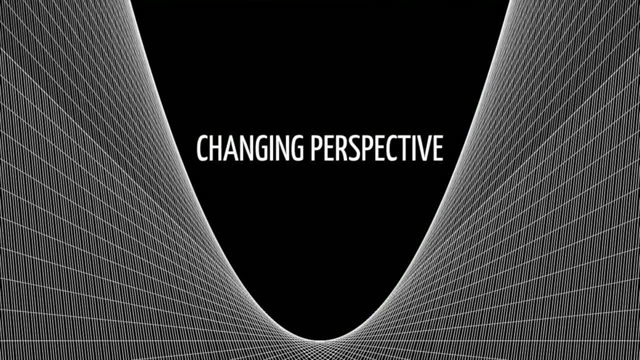 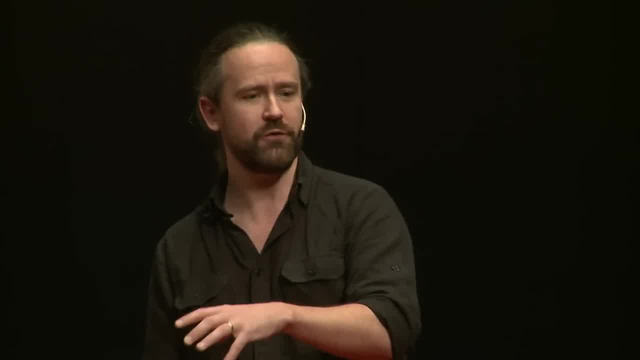 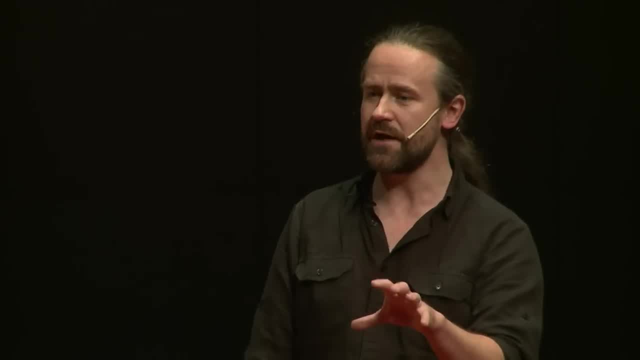 with the ability to change your perspective, And I claim that when you change your perspective and if you take another point of view, you learn something new about what you are watching or looking at or hearing, And I think this is a really important thing that we do all the time. 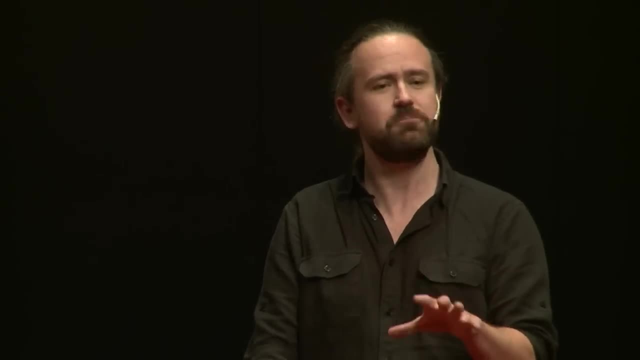 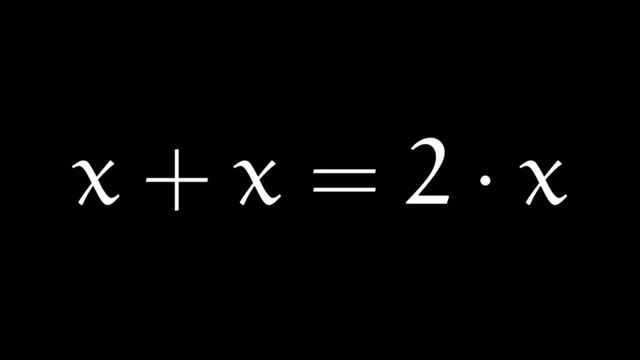 So let's just look at this simple equation like x plus x equals two times x. This is a very nice pattern And it's true, because five plus five equals two times five, et cetera, And we've seen this over and over and we represent it like this. But think about it. 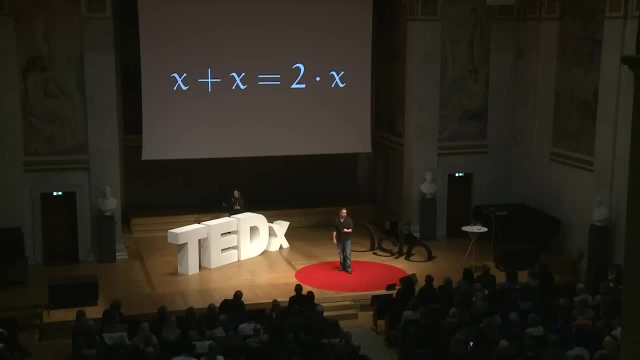 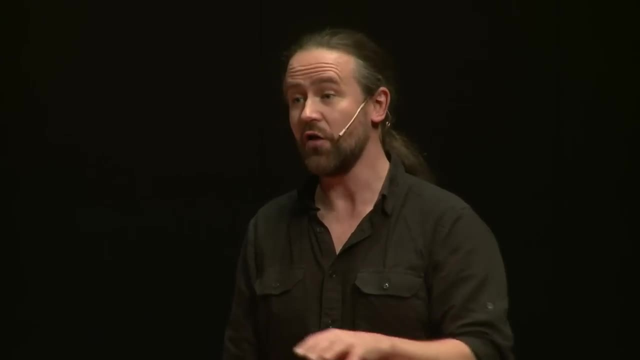 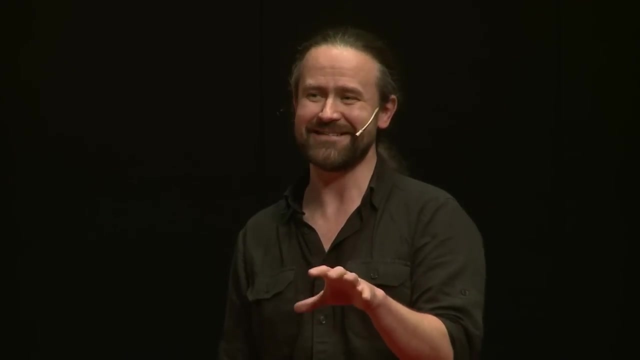 This is an equation. It says that something is equal to something else, And that's two different perspectives. One perspective is: it's a sum, It's something you plus together. On the other hand, it's a multiplication. And those are two different perspectives, And I would go as far as to say that 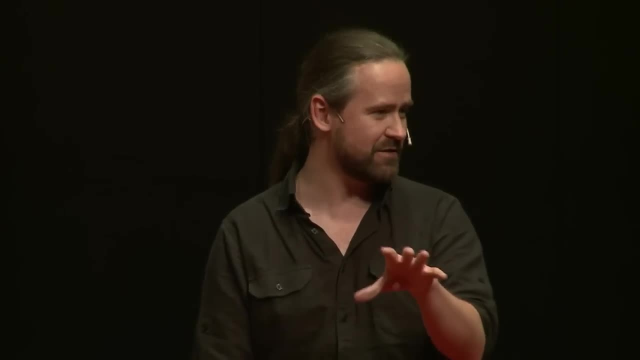 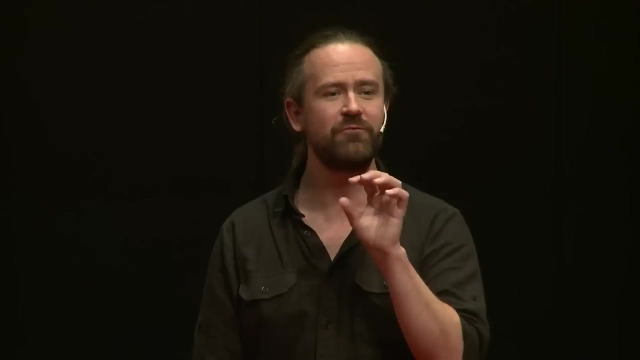 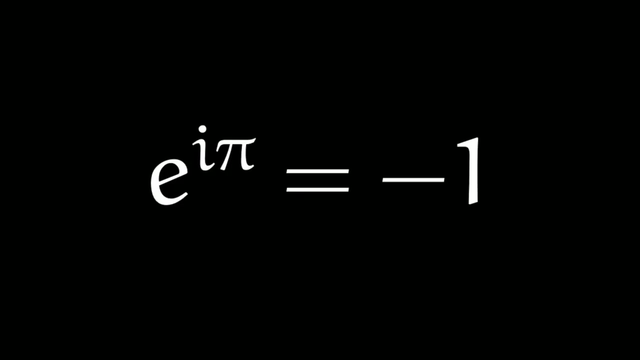 every equation is like this. Every mathematical equation Where you use that sign, that equality sign, is actually a metaphor. It's an analogy between two things: You're just viewing something and taking two different points of view, And you're expressing that in the language. Have a look at this equation. This is one of the most beautiful equations. 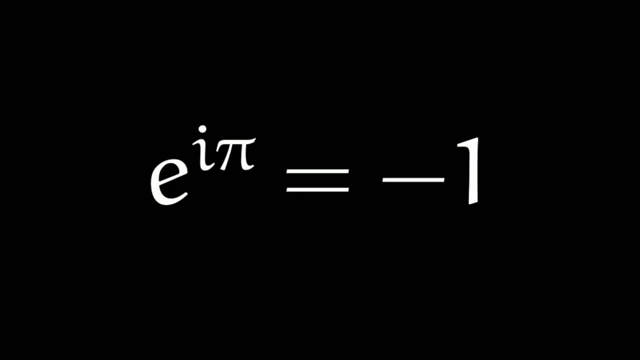 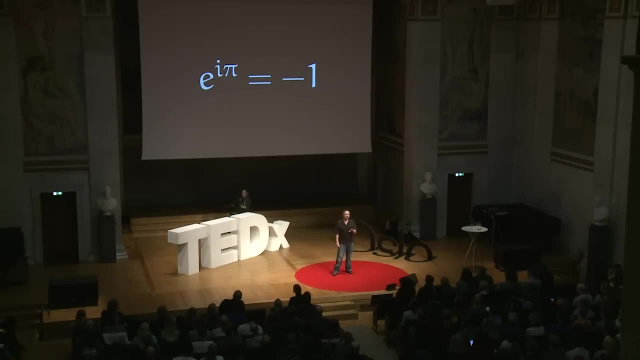 And it simply says that, well, two things. they're both negative one. This thing on the left-hand side is negative one and the other one is, And that, I think, is one of the essential parts of mathematics. You take different points of view. 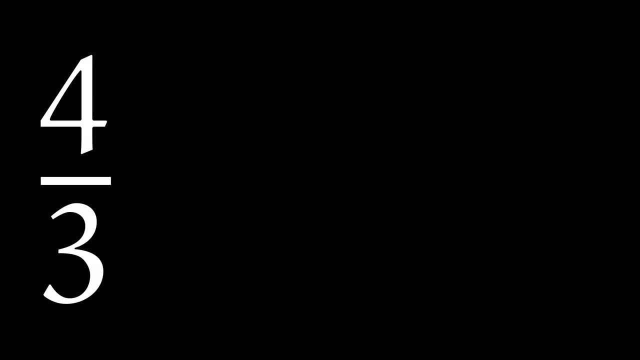 So let's just play around. Let's take a number. You know, we know four thirds, We know what four thirds is: It's 1.333.. But we have to have those three dots, Otherwise it's not exactly four. 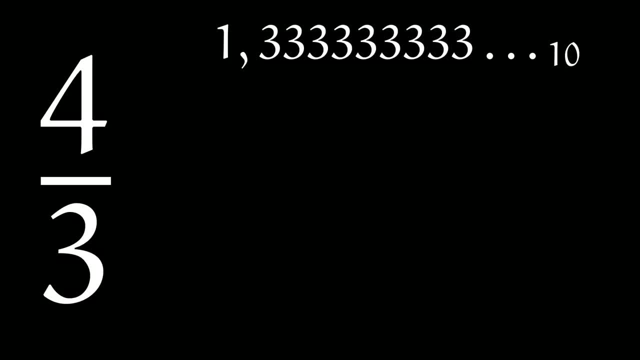 thirds. But this is only in base 10.. You know the number system. we use 10 digits. If we change that around and only use two digits, that's called the binary system. It's written like this. So we're. 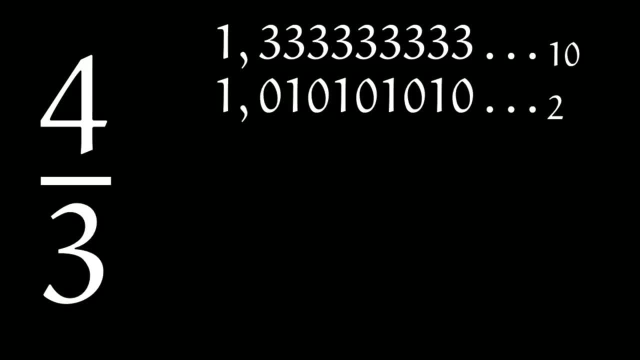 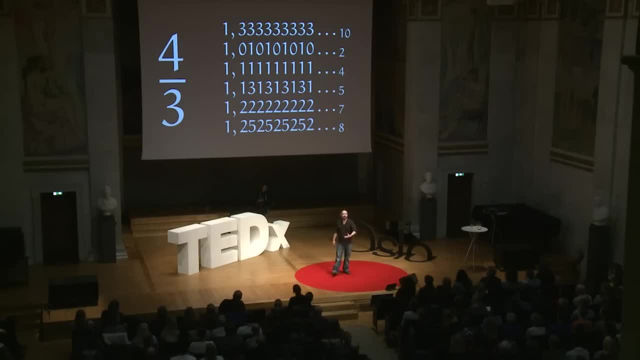 now talking about the number. The number is four thirds And we can write it like this: And we can just change the base, change the number of digits. And we can write it like this And we can just write it differently. So these are all representations of the same number. We can even 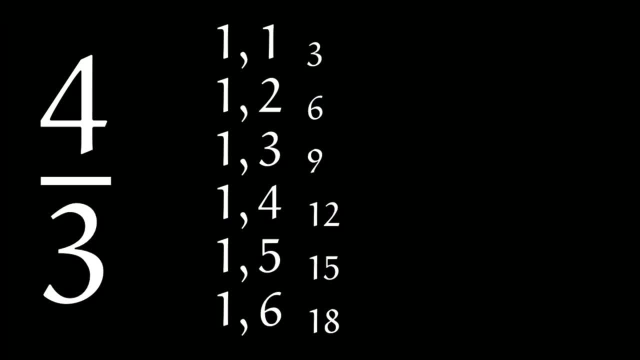 write it simply like 1.3 or 1.6.. It all depends on how many digits you have. Or perhaps we should simplify and just write it like this: I like this one because this is four divided by three And this number expresses a relation between two numbers. You have four on the one hand and three. 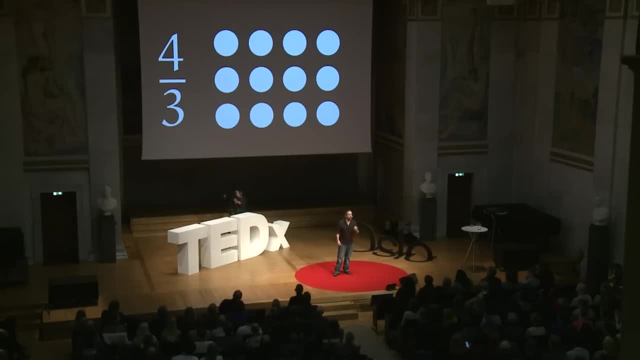 on the other, And you can visualize this in many ways, And what I'm doing now is I'm viewing that in different perspectives. I'm playing around. I'm playing around with how we view something And I'm doing it very deliberately. We can take a grid If it's four across and three up this line. 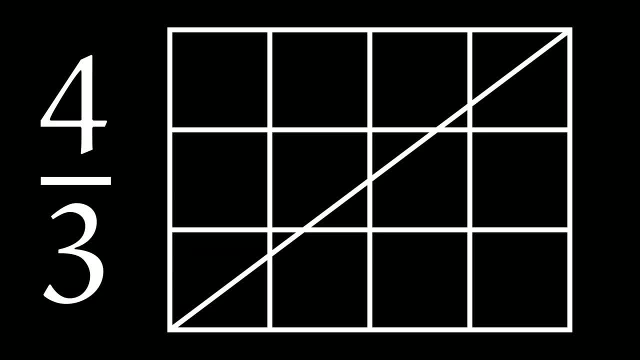 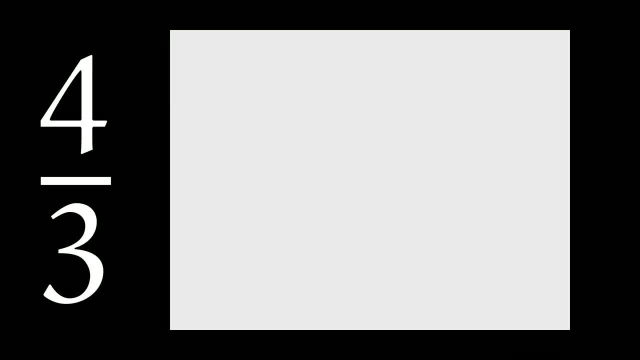 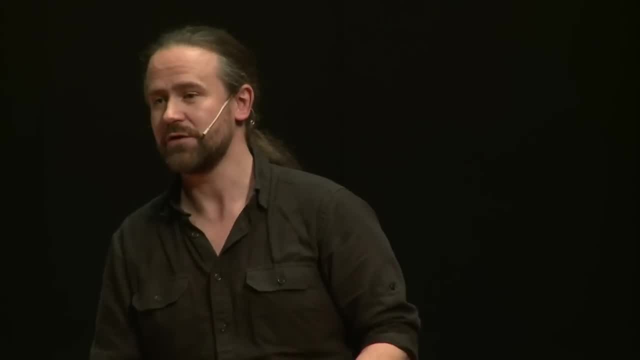 equals five. always It has to be like this. This is a beautiful pattern: Four and three and five And this rectangle which is four by three. you've seen a lot of times. This is your average computer screen: 800 by 600 or 1600 by 1200 is the television or the computer screen? 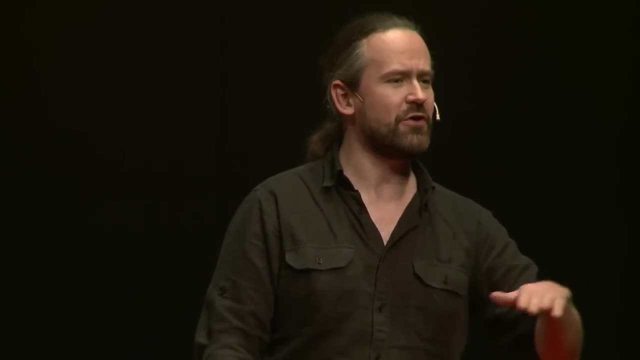 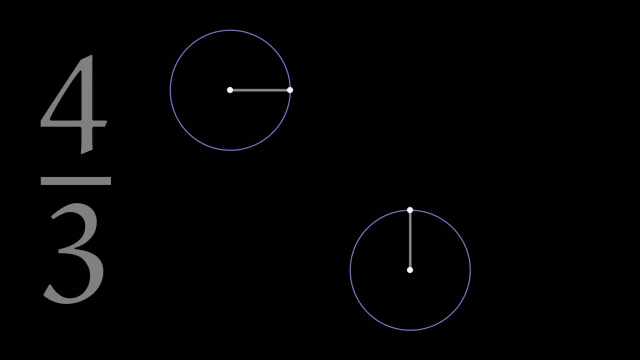 These are all nice representations, But I want to go a little bit further and just play more with this number. Here you see two circles, And I'm going to rotate them like this And observe the upper left one. It goes a little bit faster. right You can see this And it actually goes exactly. 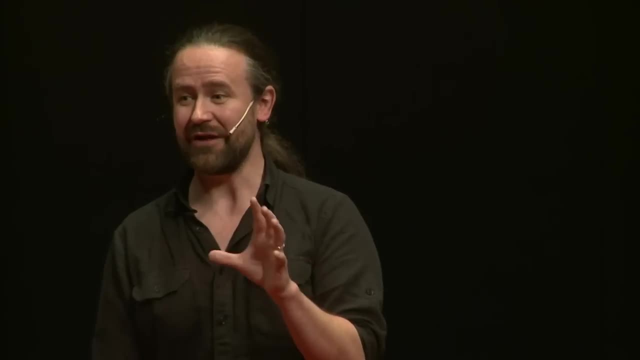 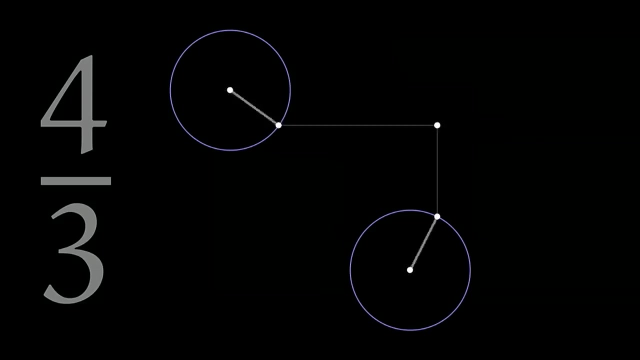 four thirds as fast, And that means that when it goes around four times, the other one goes around three times. Now let's make two lines and draw this dot where the lines meet. We get this dancing right Now. we should trace it. Let's trace it and see what happens. This is what mathematics is. 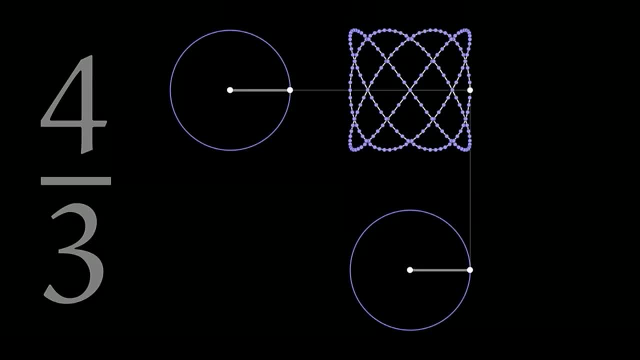 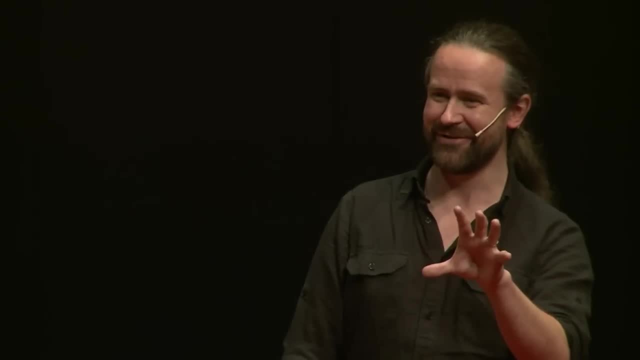 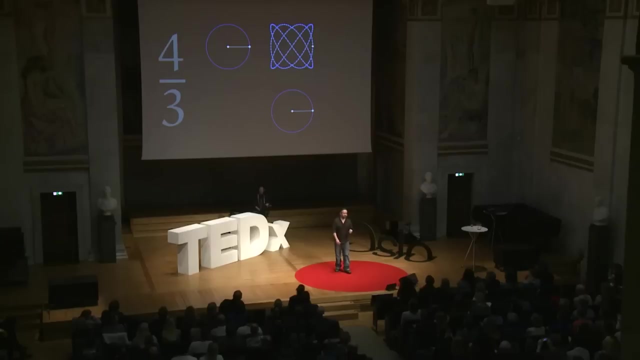 all about. It's about seeing what happens, And this emerges from four thirds. I like to say that this is the image of four thirds. It's very much nicer, Thank you, And this is not new. This has been known for a long time. 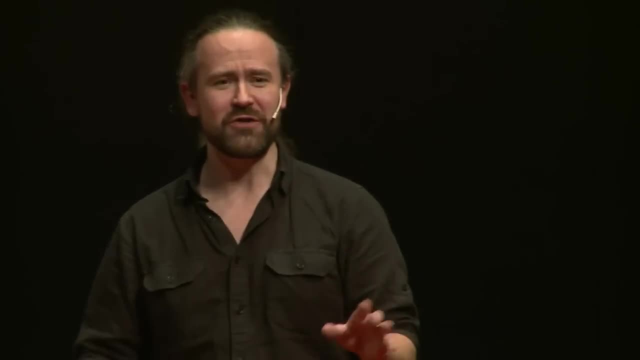 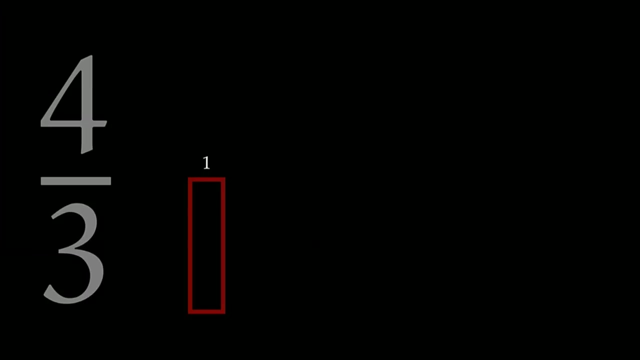 But this is four thirds. Four thirds. Let's do another experiment. Let's now take a sound, This sound, This is a perfect A 440 hertz. Let's multiply it by two, We get this sound And we play them together. Sounds like: 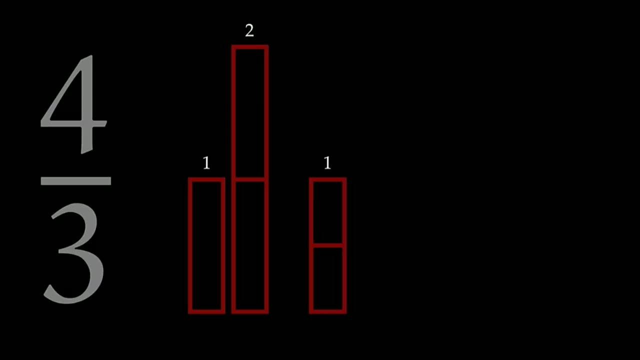 this. It's an octave. right, I can do this game. We can play a sound, play the same A. We can multiply it by three halves. This is what we call a perfect fifth. Sounds really nice together. Let's multiply this sound by four thirds. 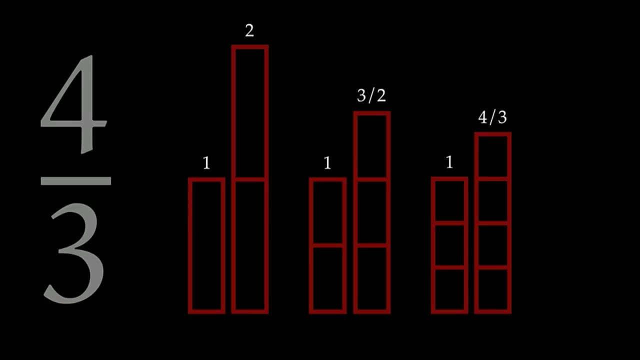 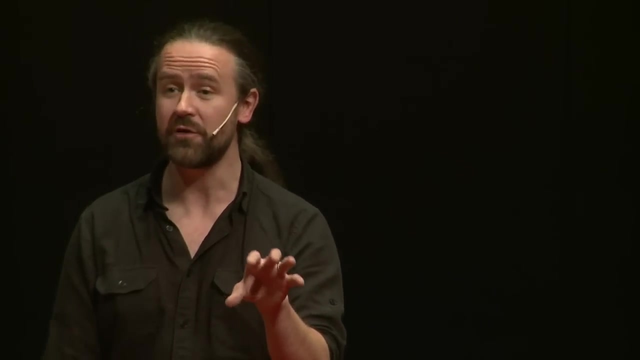 Four thirds. right, What happens? You get this sound. This is the perfect fourth. If the first one is an A, this is a D. They sound like this together. This is the sound of four thirds. What I'm doing now, I'm changing my perspective. I'm just viewing a number from another perspective. 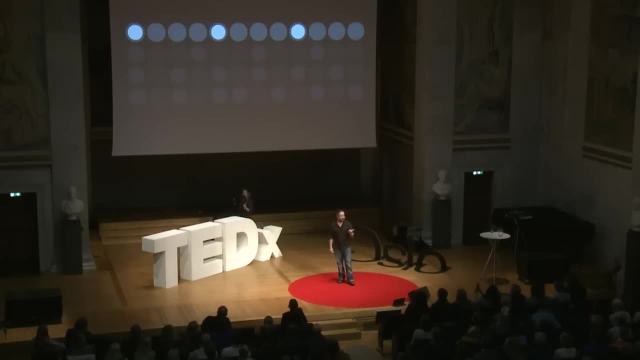 I can even do this with rhythms, right, I can take a rhythm and play three beats at one time in a period of time, And I can play another sound four times in that same space. Okay, It sounds kind of boring, but listen to them together. 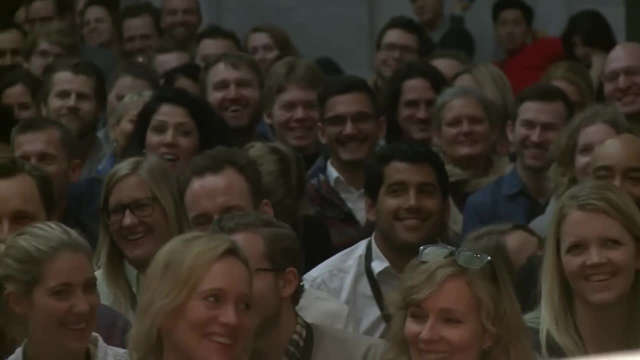 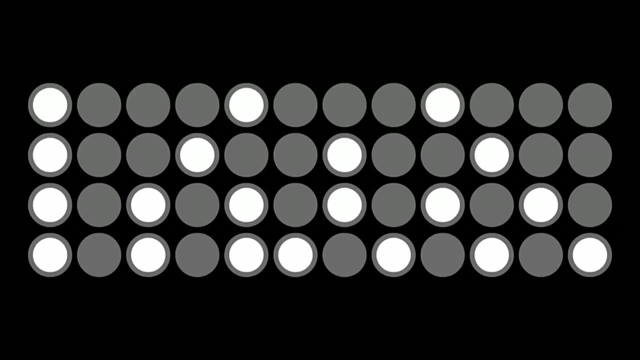 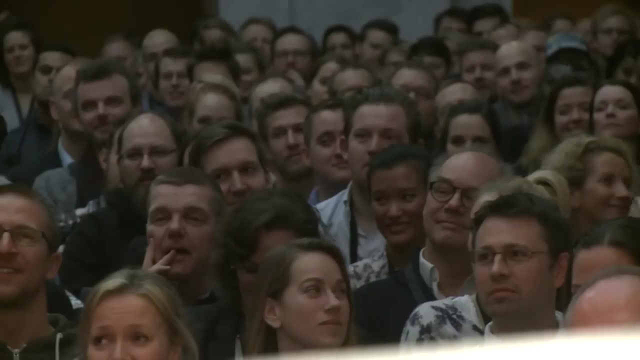 Hey, So I can even make you make a little hi-hat, Can you hear this? So this is the sound of four thirds Again. this is as a rhythm, And I can keep doing this and play games with this number. Four thirds is a really great number. I. 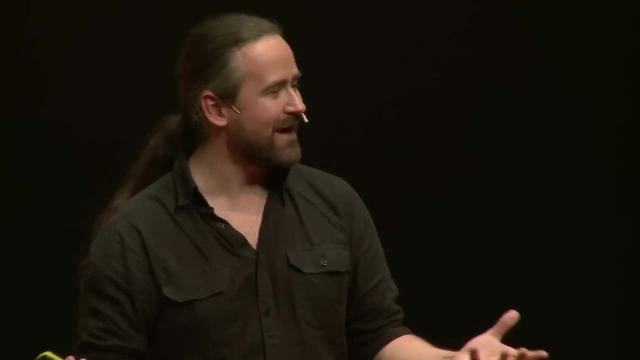 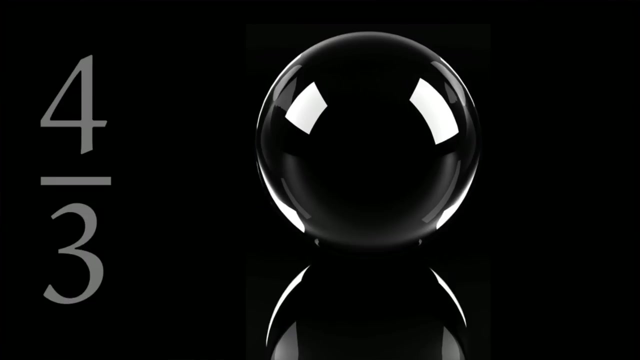 love. four thirds. I mean truly Undervalued number. So if you take a sphere and look at the volume of the sphere, it's actually four thirds of some particular cylinder. So four thirds is in the sphere. It's the volume of the. 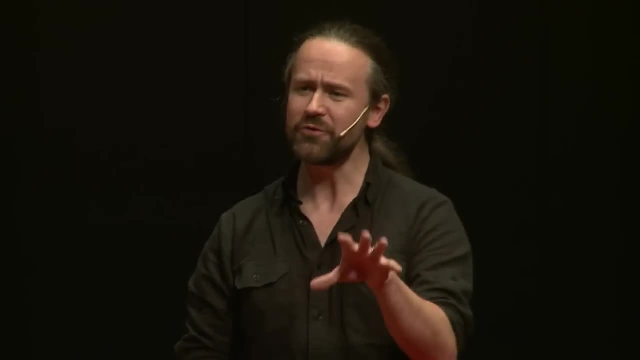 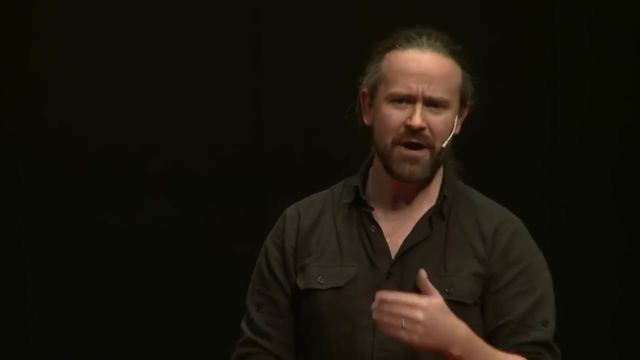 sphere. Okay, So why am I doing all this? Well, I want to talk about what it means to understand something, And what do we mean by understanding something? That's my aim here, And my claim is that you understand something if you have the ability to view it from different perspectives. 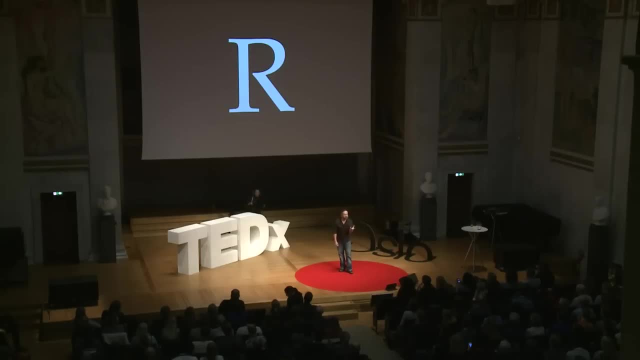 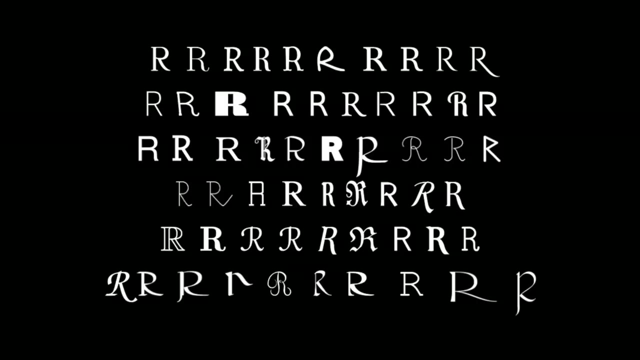 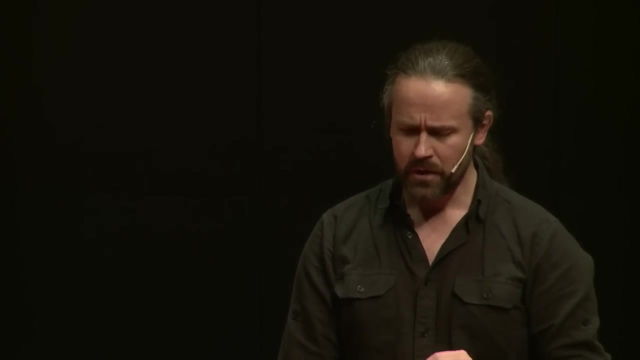 Let's look at this letter. It's a beautiful R, right? How do you know that? Well, as a matter of fact, you've seen a bunch of R's and you've generalized it and abstracted over all these and you found the pattern. So you know that this is an R. So what I'm aiming for here is: 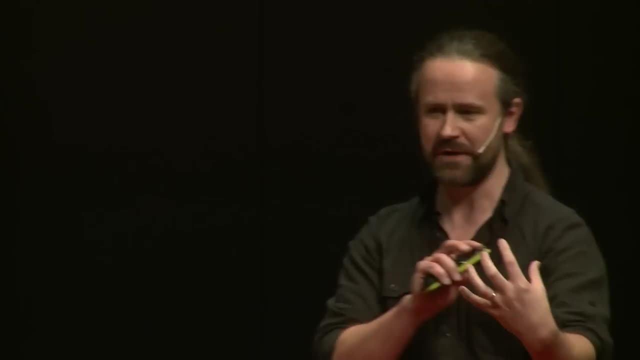 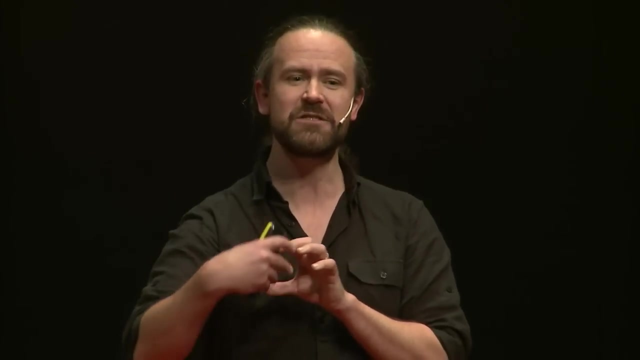 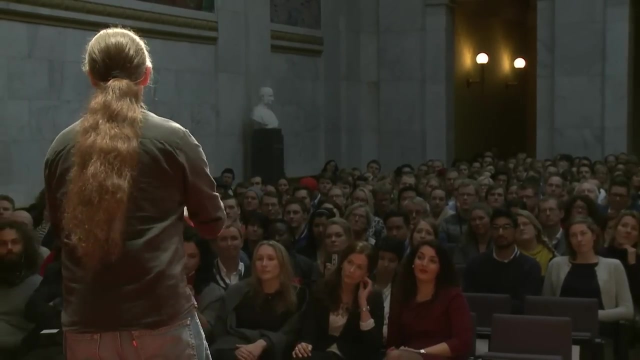 saying something about how understanding and changing your perspective is linked. And I'm a teacher and I'm a lecturer and I can actually use this to teach something, because when I give someone else another story, a metaphor, an analogy, if I tell a story from a different point of view, I enable understanding, I make understanding. 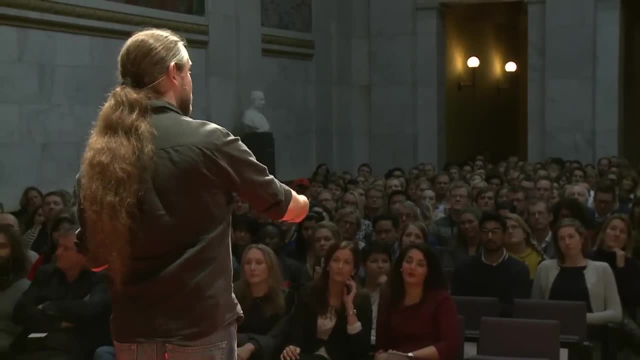 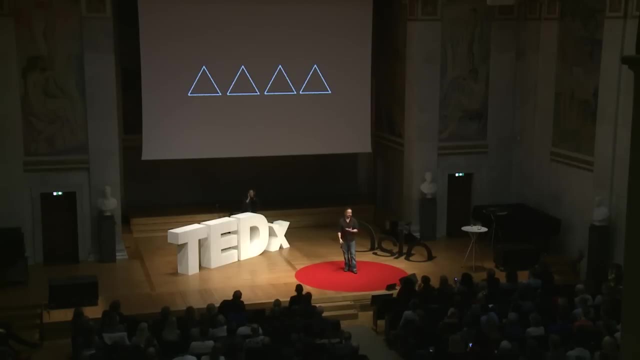 possible, because you have to generalize over everything you see and hear, And if I give you another perspective, that will become easier for you. Let's do a simple example again. This is four and three, This is four triangles, So this is also four thirds in a way. Let's just join them. 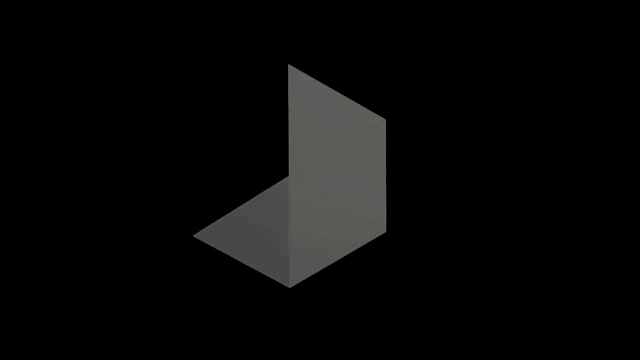 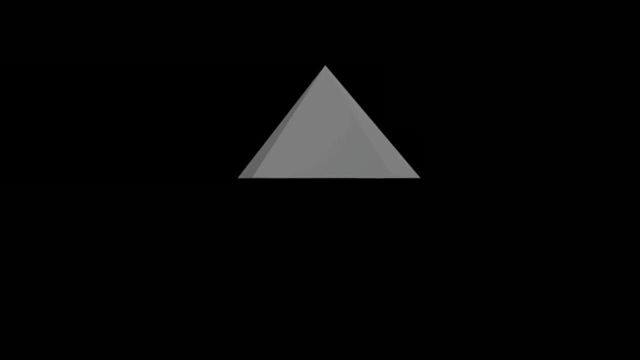 together. Now we're going to play a game. We're going to fold it up into a three-dimensional structure. I love this. This is a square pyramid, Okay, And let's just take two of them and just put them together, Okay. So this is what is called the. 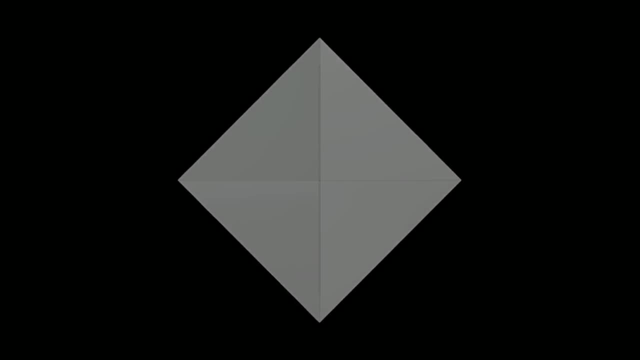 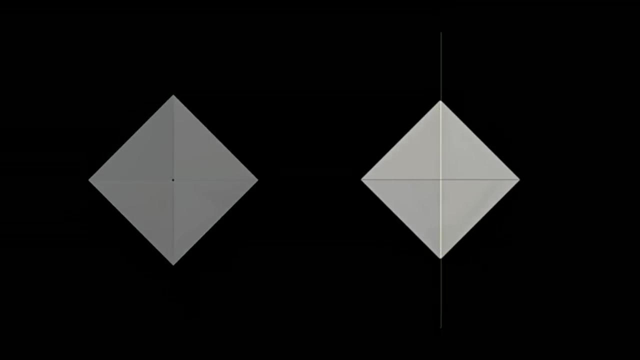 octahedron. It's one of the five platonic solids. Now we can quite literally change our perspective, because we can rotate around one of the axes and view it from different perspectives, And I can change the axis and then I can view it from another point of view, But it's the same thing. 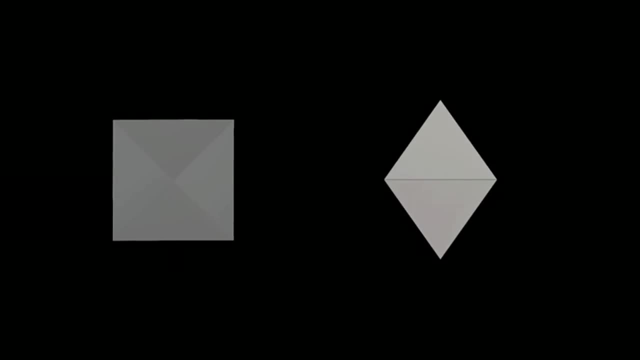 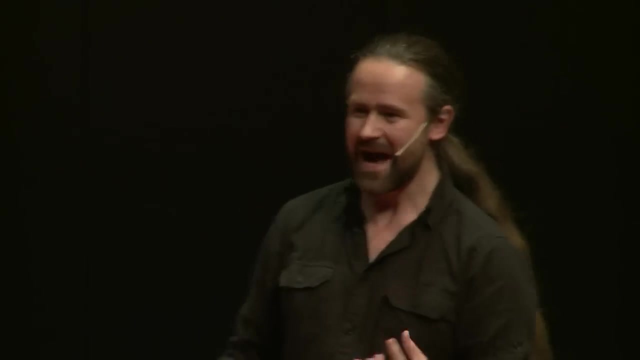 but it looks a little bit different And I can do it even one more time. Every time I do this, something else appears, So I'm actually learning more about the object. when that changed my perspective. I can use this as a tool for creating understanding. 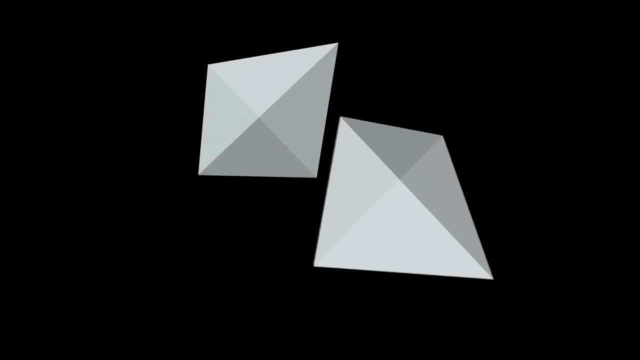 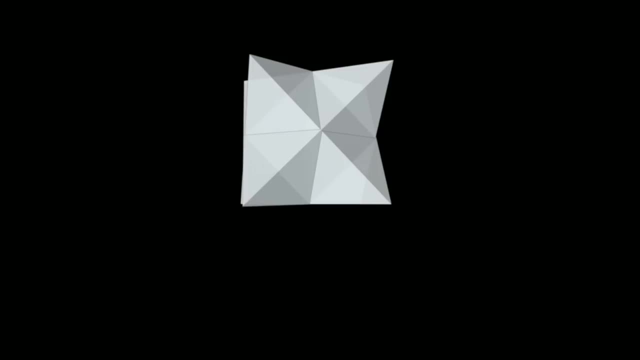 I can take two of these and just put them together like this and see what happens, And it looks a little bit like the octahedron. Have a look at it. If I spin it around like this, what happens? Well, if you take two of these, join them together and spin it around, 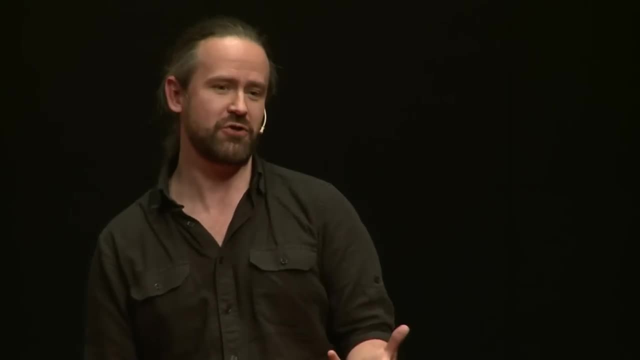 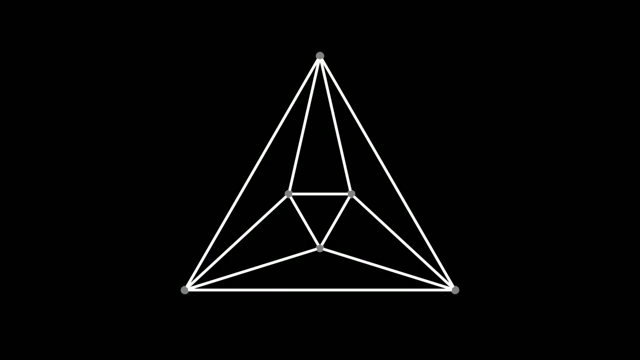 there's your octahedron Again, a beautiful structure If you lay it out flat on the floor. this is the octahedron. It's a graph structure of an octahedron, And I can continue doing this. You can draw three. 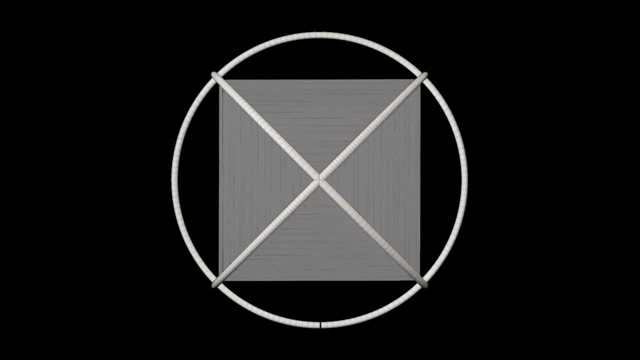 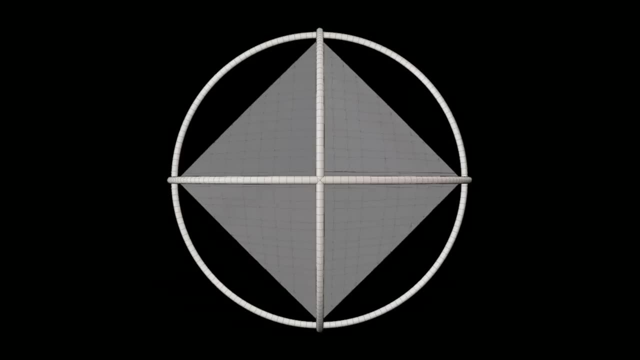 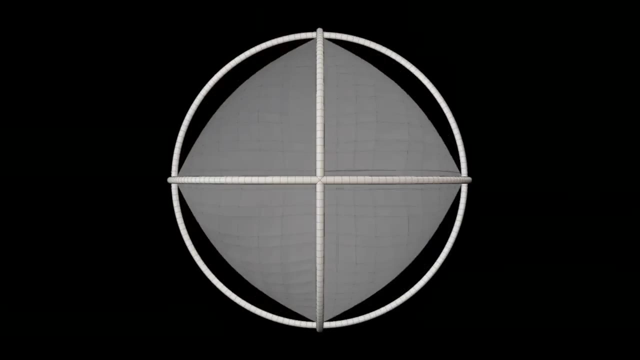 great circles around the octahedron and rotate around. So actually three great circles is related to the octahedron And if you take a bicycle pump and just pump it up, you can see that this is also a little bit like the octahedron. Do you see what I'm doing here? I am changing the 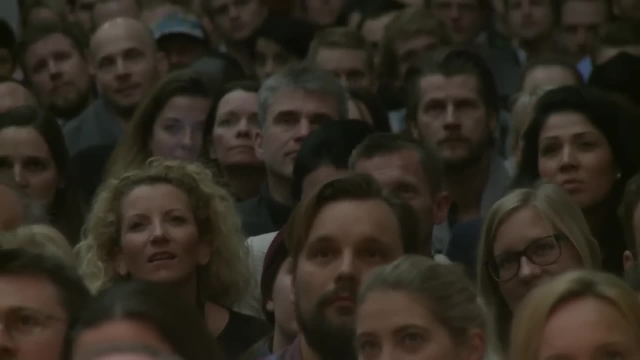 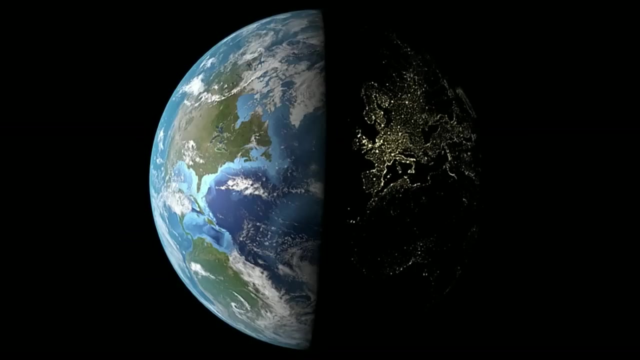 perspective all the time, But take a step back- And that's actually a metaphor: Stepping back And have a look at what we're doing. I'm playing around with metaphors, I'm playing around with perspectives and analogies. I'm telling one story in different ways. I'm telling stories, I'm making a narrative And I'm 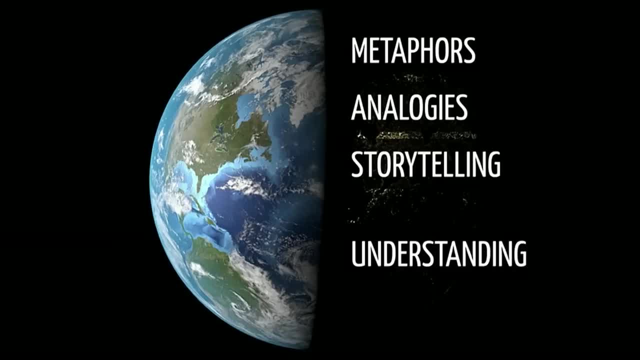 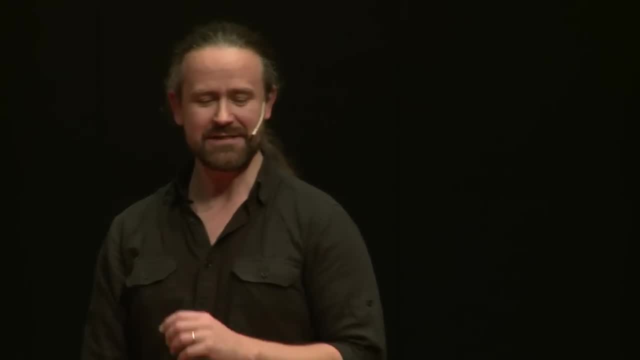 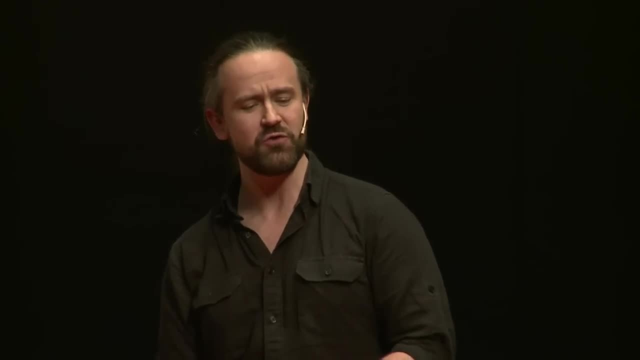 making several narratives, And I think all these things makes understanding possible. I think this actually is the essence of understanding something And I truly believe this. So this thing about changing your perspective, it's absolutely fundamental. It's fundamental for humans. Let's play around with this earth. Let's zoom into the ocean. Have a look at the ocean. 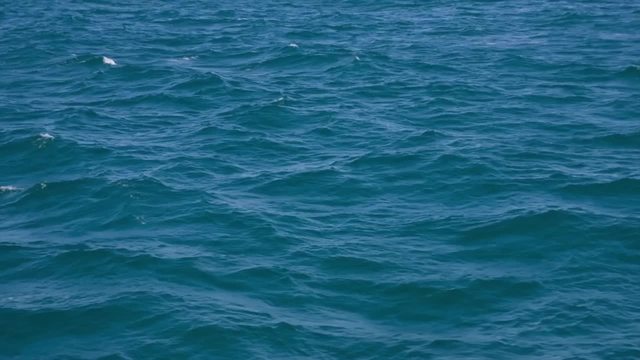 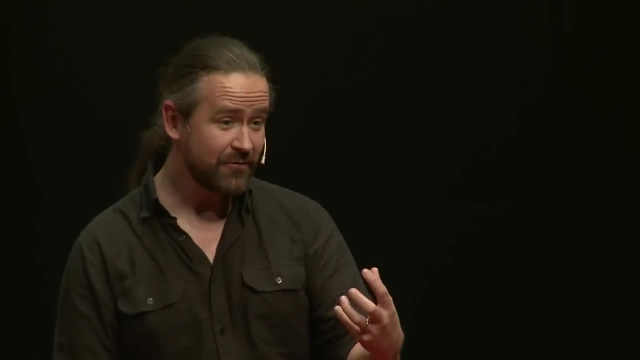 We can do this with anything. We can take the ocean and view it up close. We can look at the waves. We can go to the beach. We can view the ocean from another perspective. Every time we do this, we learn a little bit more. 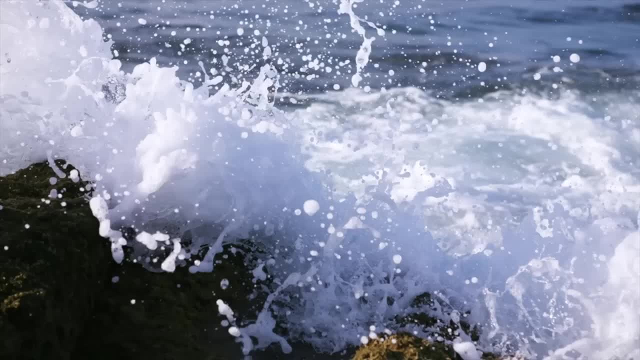 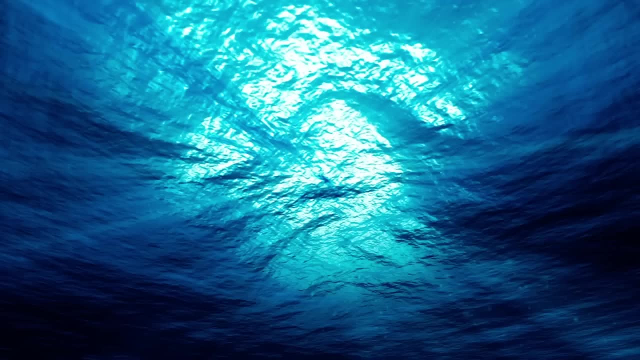 about the ocean. If we go to the shore, we can kind of smell it right. We can hear the sound of the waves, You can feel the salt on our tongues. So all these are different perspectives And this is the best one We can go. 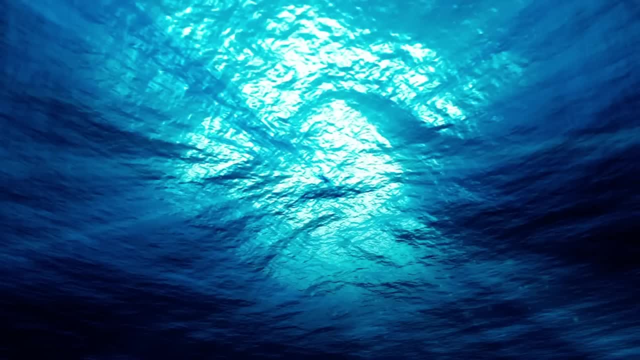 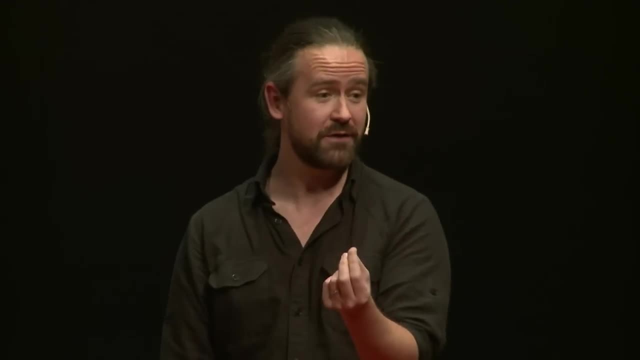 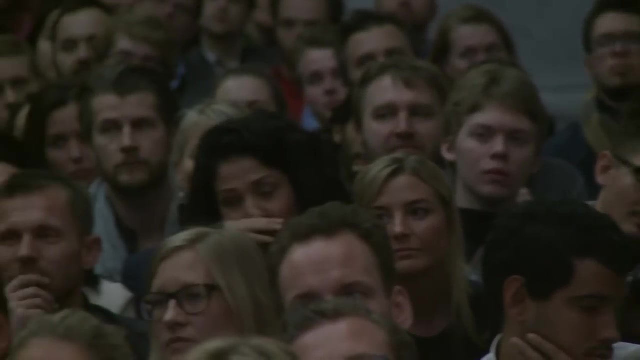 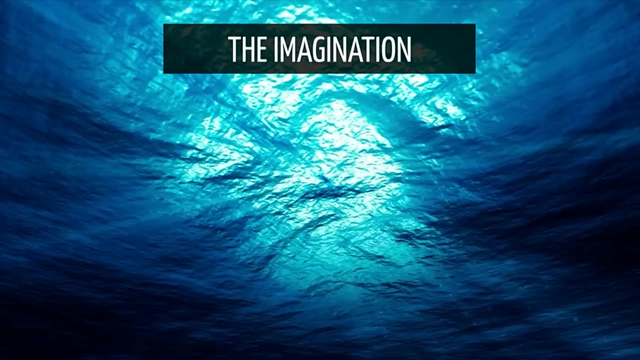 the inside, then you really learn something about it. That's somehow the essence of something. So when we do this- and we've taken this journey into the ocean- we use our imagination, And I think this is one level deeper And it's actually a requirement for changing your perspective. 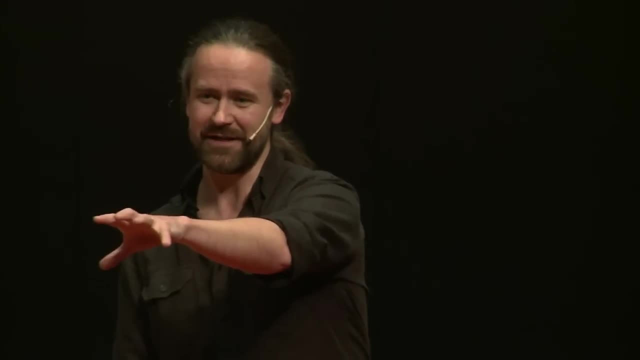 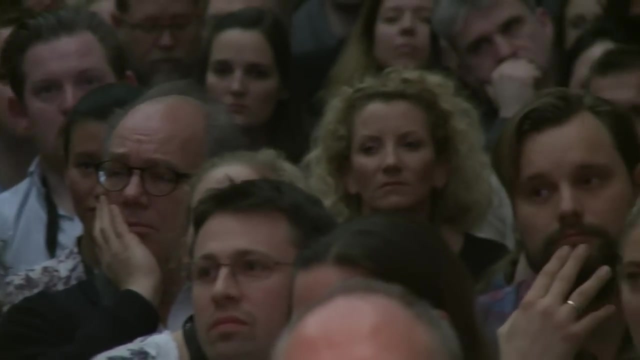 We can do a little game. You can actually imagine that you're sitting there. You can imagine that you're up here and that you're sitting here, You can view yourself from the outside. That's really a strange thing. You're changing your perspective, You're using your imagination And you're reviewing. 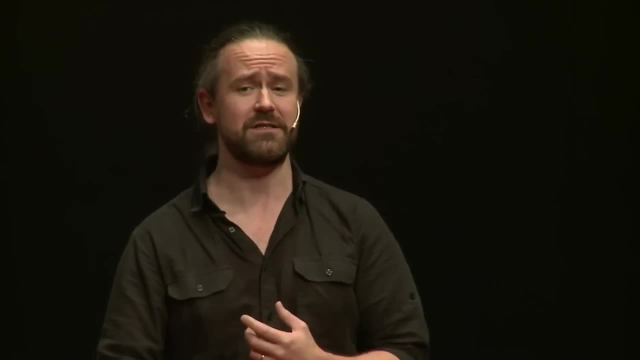 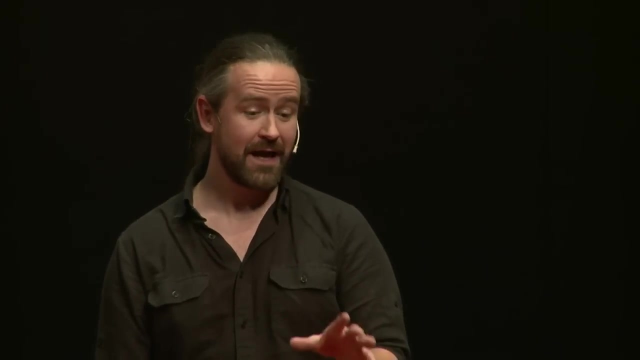 yourself from the outside, And that requires imagination And mathematics and computer science is the most imaginative art forms ever, And this thing about changing perspectives should sound a little bit like this, Because we do it every day, And then it's called empathy. When I view the 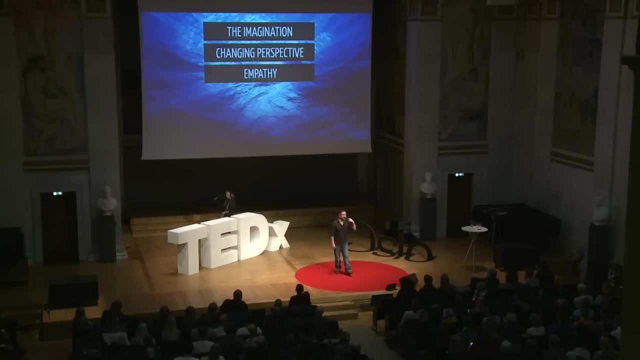 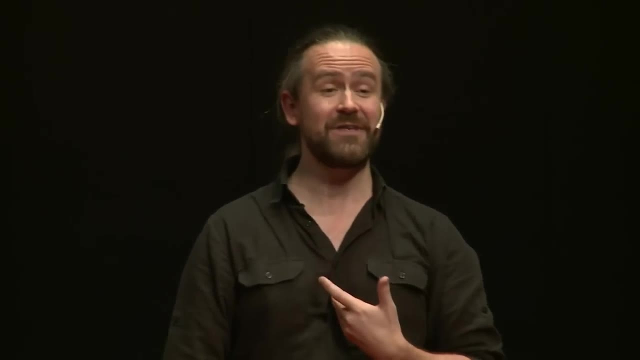 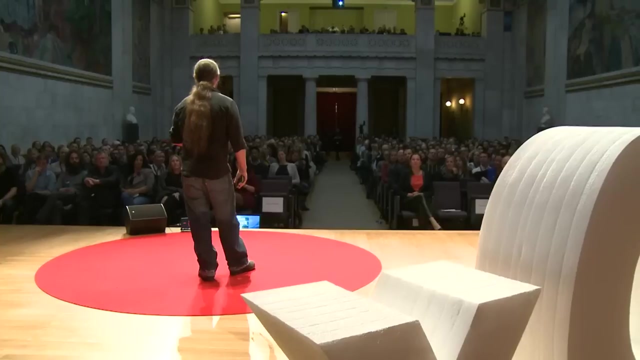 world from your perspective. I have empathy with you. If I really truly understand what the world looks like from your perspective, I am empathetic. That requires imagination And that is how we obtain understanding. And this is all over mathematics And this is all over computer.